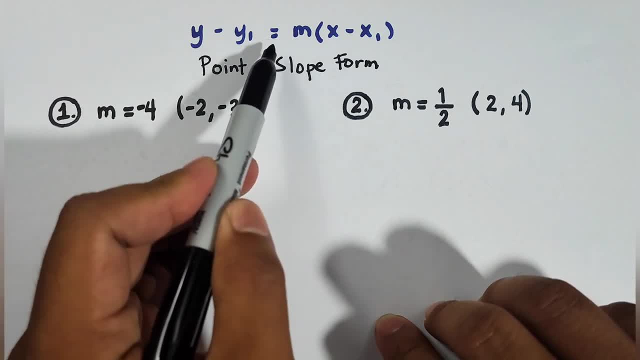 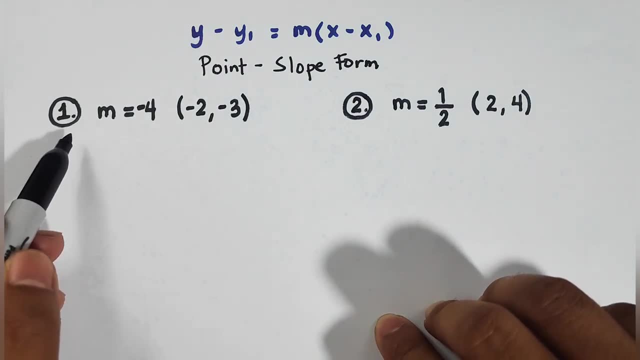 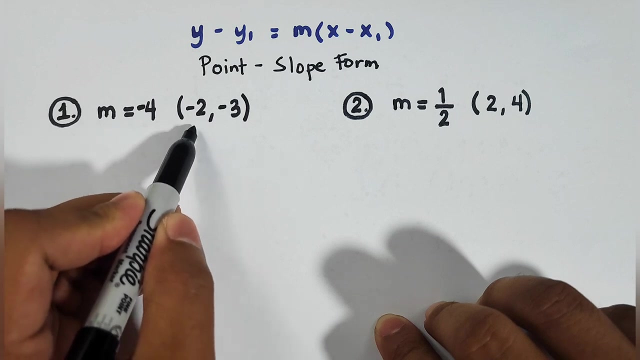 Here the variable m represents the slope, x sub 1 and y sub 1 are the coordinates of your point. So let's solve and find the equation of number 1.. m is equal to negative 4 and the coordinates of the single point is negative 2, negative 3.. So let's copy the given form: y minus y sub 1. 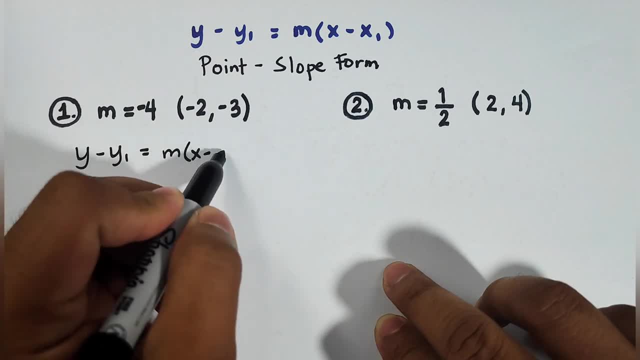 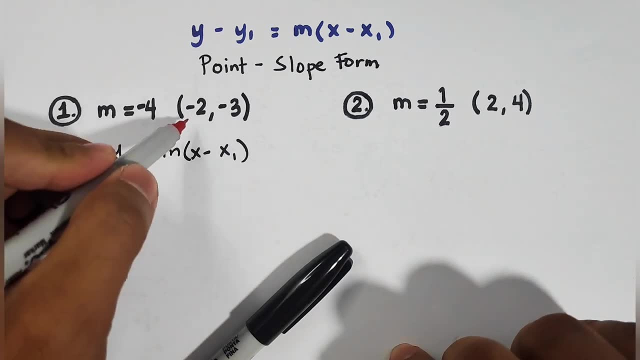 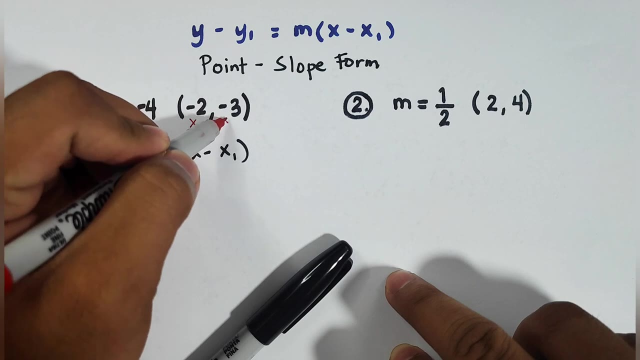 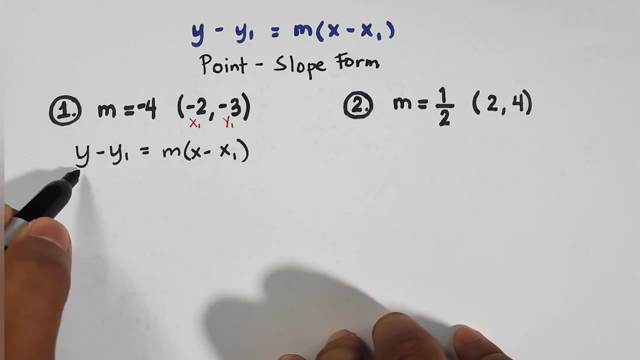 is equal to m times x minus x sub 1.. Now, guys, in this form, your negative 2 represents x sub 1.. Your negative 3, this one represents your y sub 1.. And what we need to do is to substitute the values in the given form For this variable y and variable x. 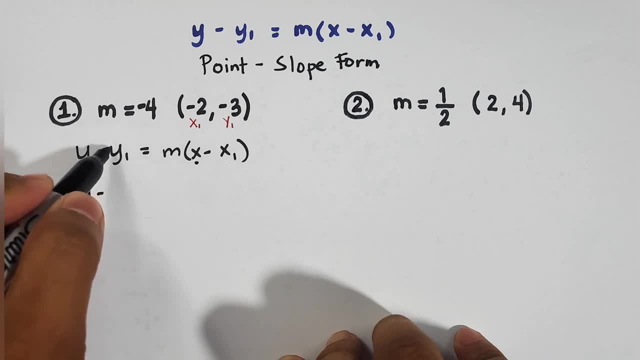 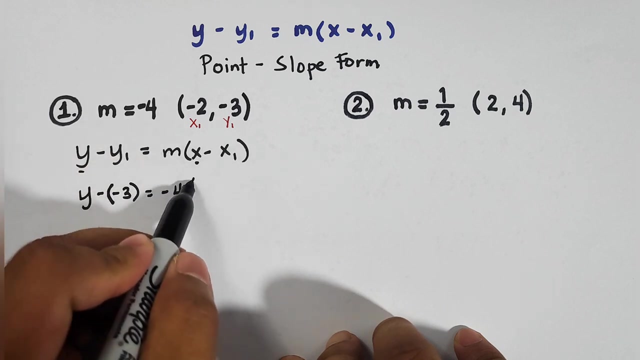 copy y, then minus Your y sub 1 is negative 3. Since this is negative, we will enclose it by a parenthesis. Then equal to your m, which is negative 4 times. this is x minus, as you can see. 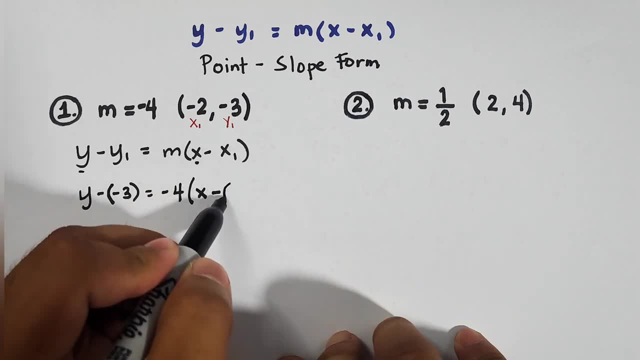 your x sub 1 is negative. 2. Enclose it by parenthesis. Okay, simplify the signs. Negative times: negative is positive, So it will become: y plus 3 is equal to negative 4. This is x sub 1.. And this one before multiplying negative 4. 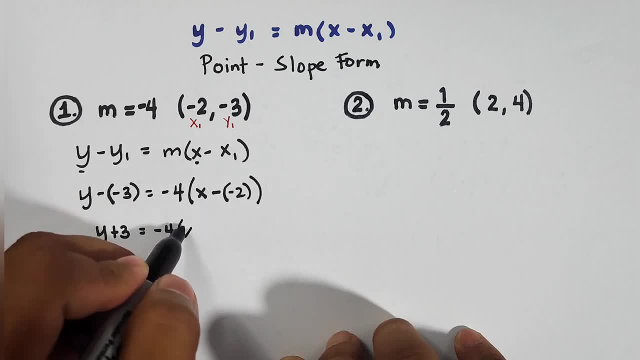 to x. then let's simplify: negative times negative, So this is times plus 2.. So, as you can see, plus 2, it came from negative times negative, And we are ready to use distributive property to multiply this. So we have: y plus 3 is equal to negative 4 times x is negative 4x. 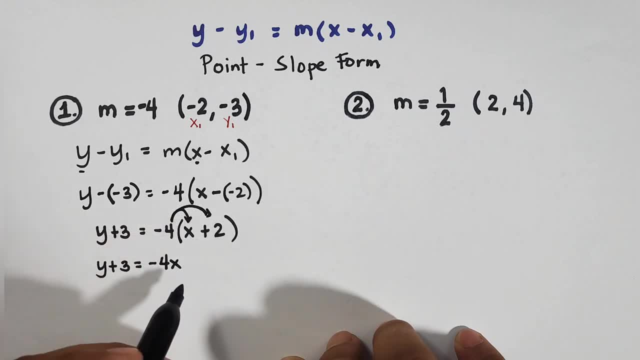 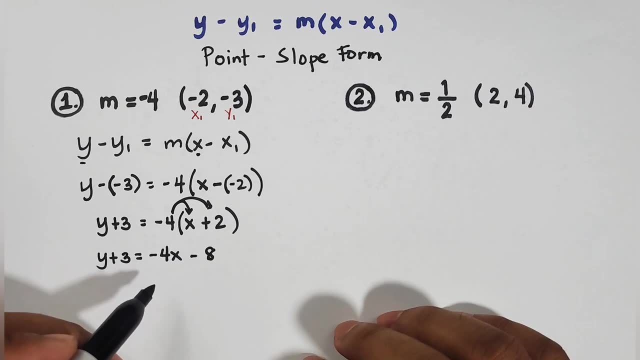 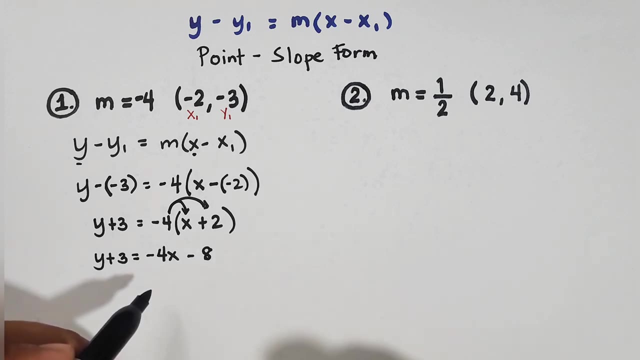 the negative 4 times 2, that is negative 8. so normally, guys, when we are doing equations of the line, we are asked to represent our answer or finalize our answer in slope intercept form and in standard form. that is what we are going to do now. here we will transpose negative 3. 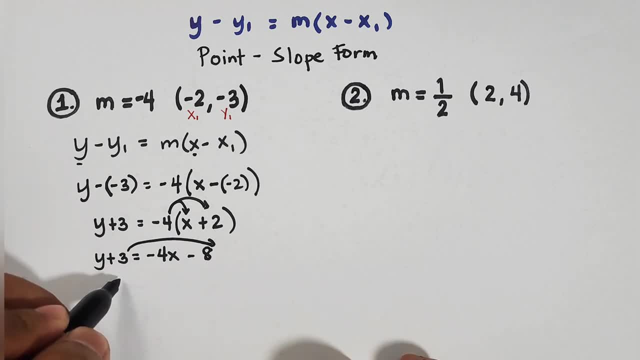 para makuha natin kanyang slope intercept form, it will become: y is equal to negative 4x minus 8 minus 3. so this is y is equal to negative 4x, this is negative 11 or minus 11 and, as you can see, 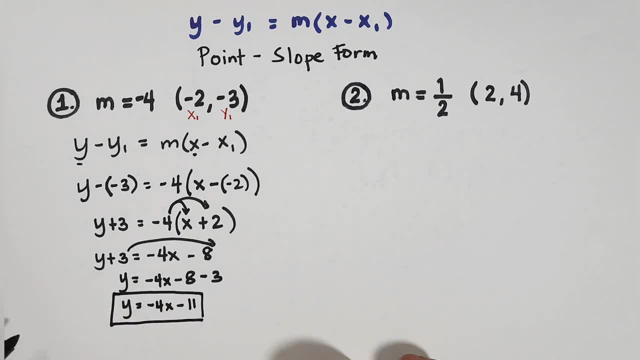 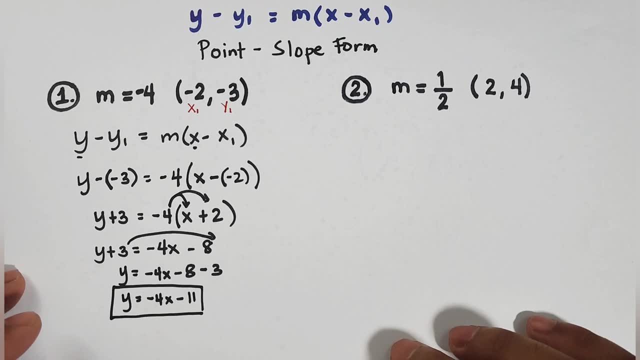 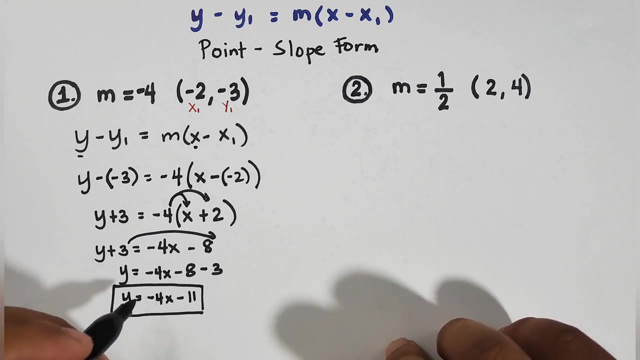 this is the slope intercept form. now let's go to the next step. so with the standard form. as for the standard form, guys, let me adjust the paper. for the standard form, we will transpose negative 4x to the other side. it will become positive 4x. so the standard form is 4x. 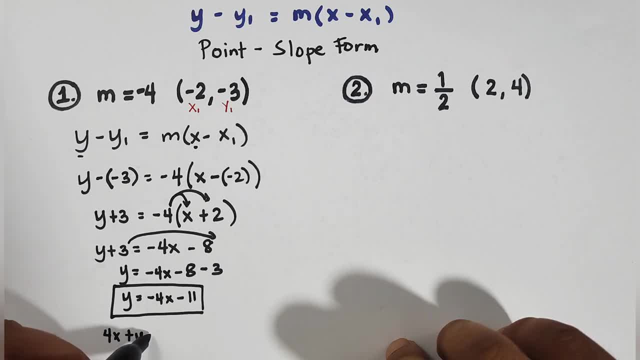 plus y is equal to negative 11. okay, these are the two forms na meron tayo, so i hope na nakuha niyo yung pattern natin on how to use the point slope form using the standard form. so let's go to the next step. 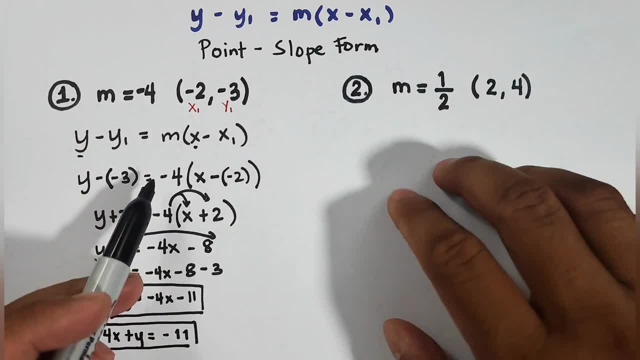 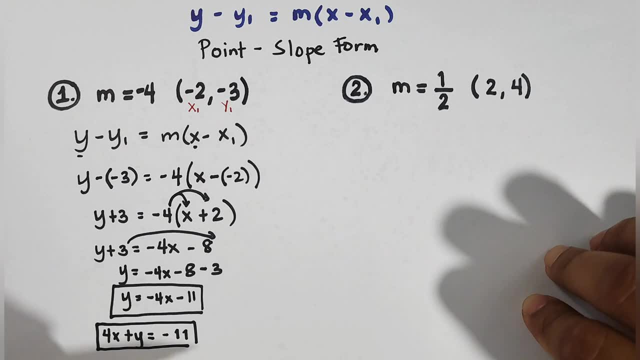 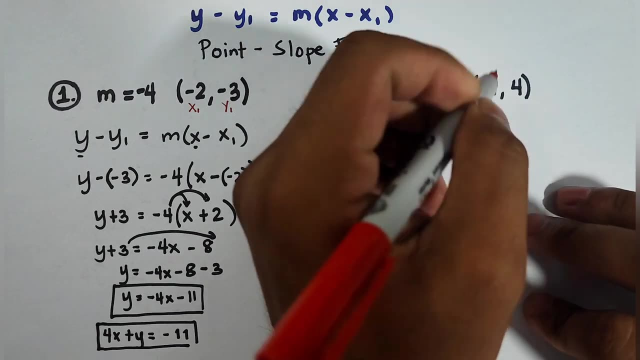 now let's move on to item number two. for number two, your m is a fraction, but don't worry kaya kaya yan. then the coordinates of the point is 2 and 4. this is your x sub 1 and this is your y sub 1. so, using the formula, let us substitute directly: 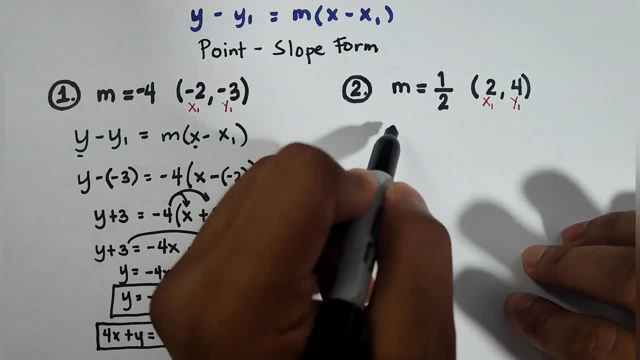 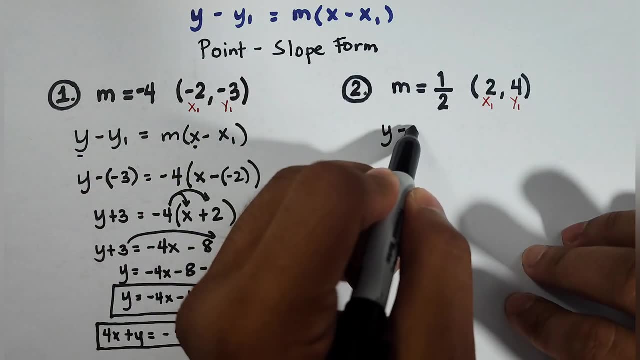 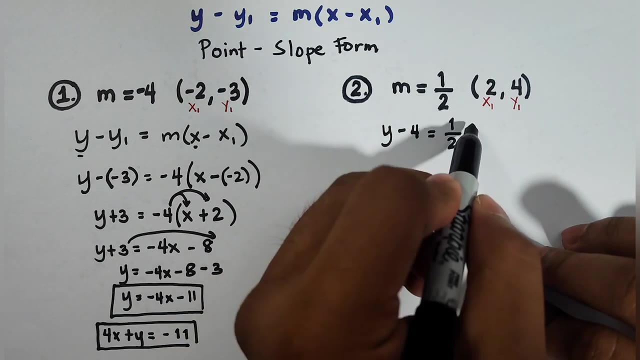 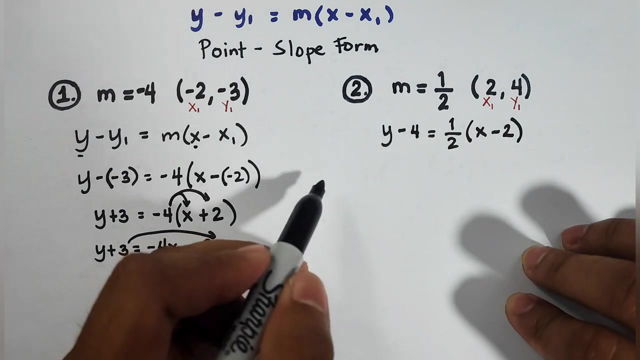 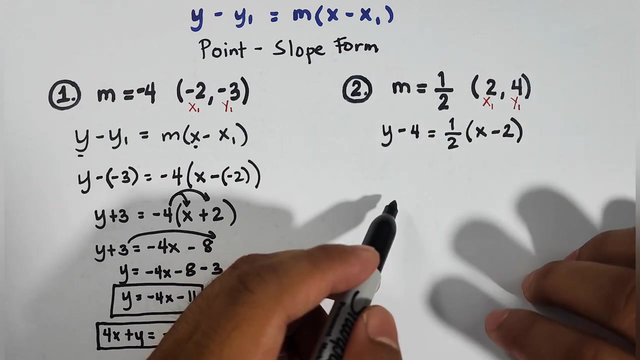 so y copy y minus your y sub 1 is 4. since that is positive, simply put, 4 is equal to one half times x minus your x sub 1, which is equal to 2. so what we need here is that there are plenty of ways on how to continue this. 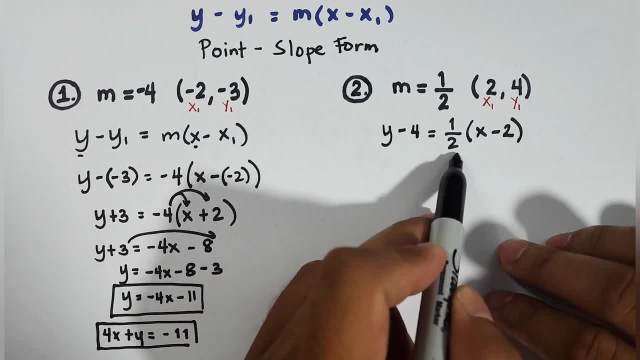 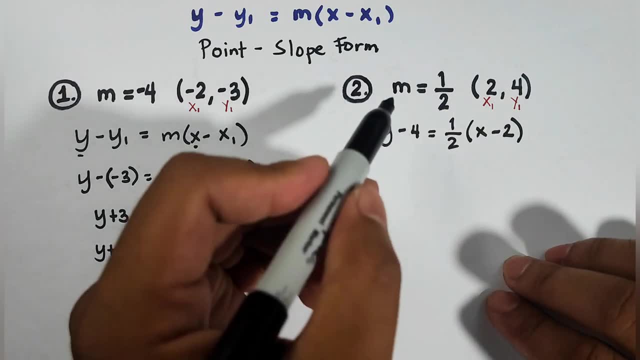 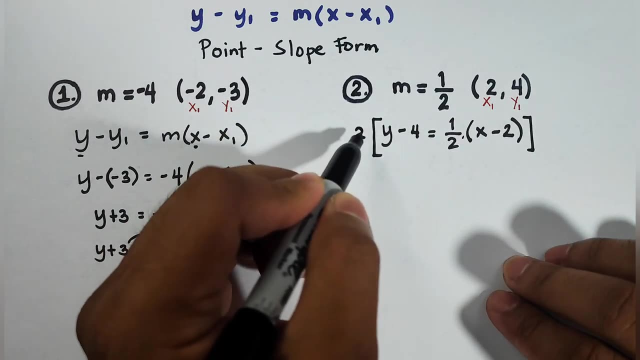 ako, what i need to do is i will eliminate first this denominator. what i need to do before doing a distributive property, i will eliminate this denominator. so i will multiply the whole equation by the denominator 2, and this is 2.. 2 times y is 2y. 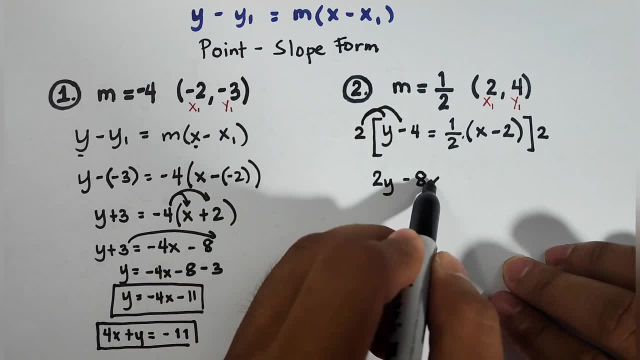 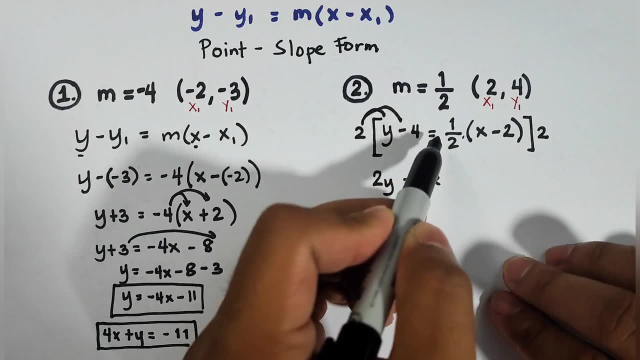 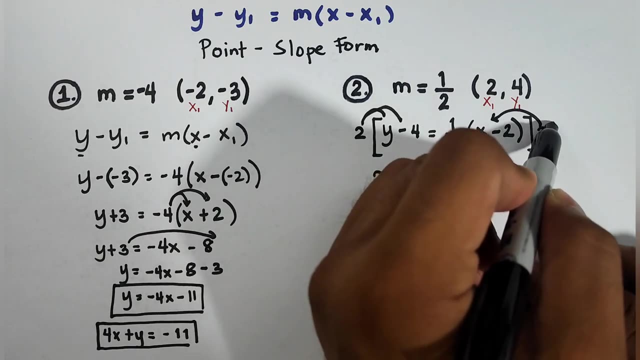 2 times negative. 4 is negative 8 and this one, this part, this part is considered as a single term. so once lang tayo mag multiply, multiply this, so kapag minultiply mo yung dito sa whole, na to makakancel na natin yung 2 and 2, so what will remain is equal to 1 times x minus 2. 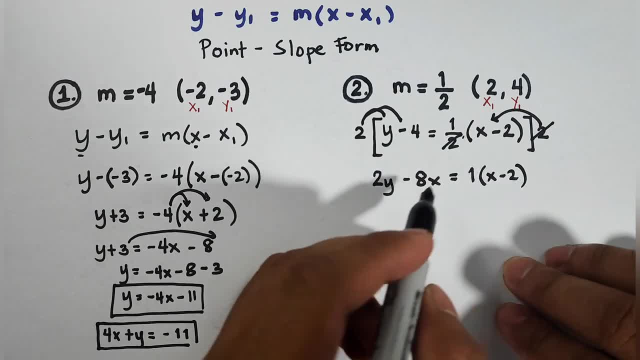 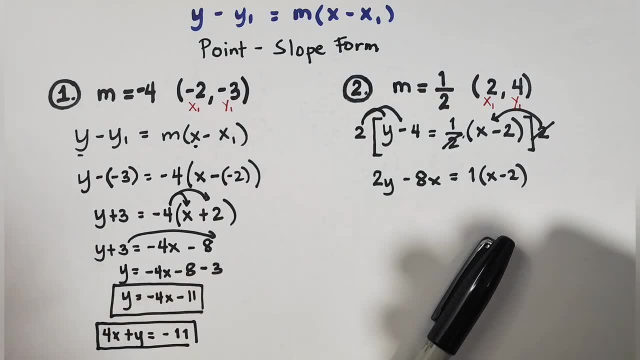 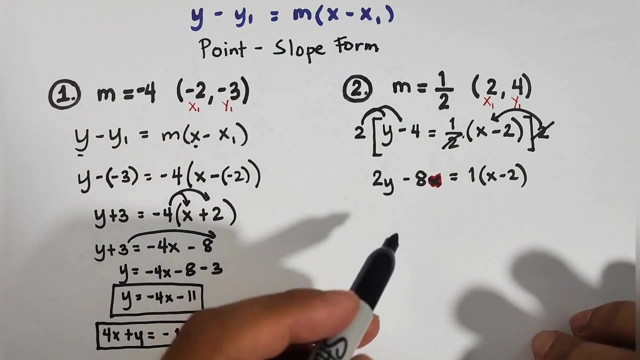 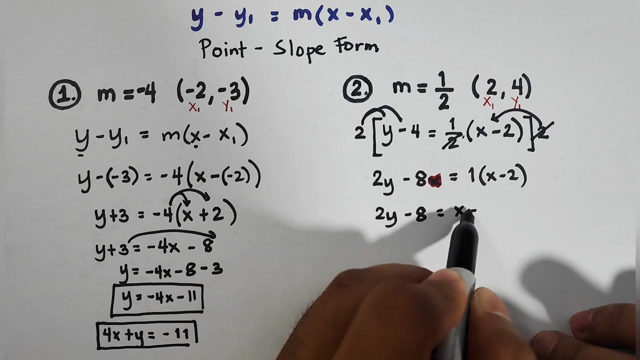 pero since 1 lang naman to this one is the same as: oh sorry, let me remove the variable x here. this is not included. ha guys, this is not included. you only have 2y minus 8, and then that is 2y minus 8 is equal to multiply 1, that is x minus 2.. What's next here? 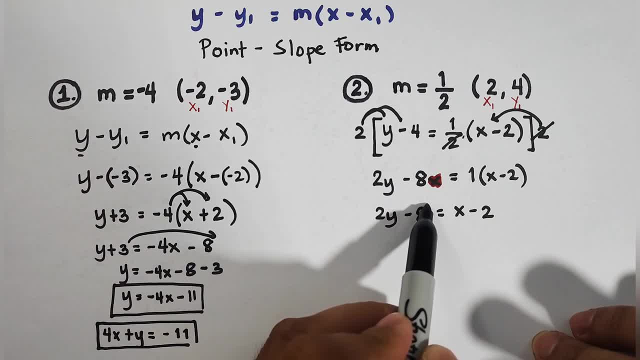 is. we will transpose this to the other side. so we have: 2y is equal to x minus 2. from negative it will become positive, so plus 8.. So this is 2y is equal to x plus 6. and to finally get the: 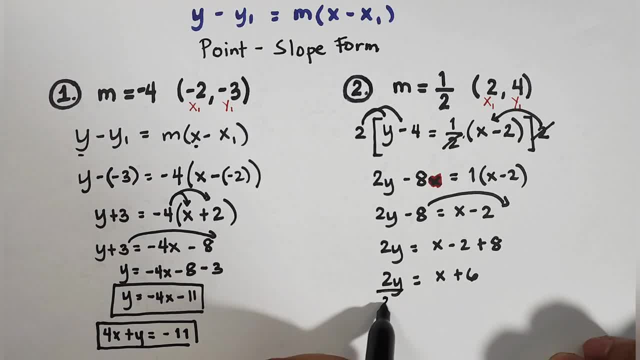 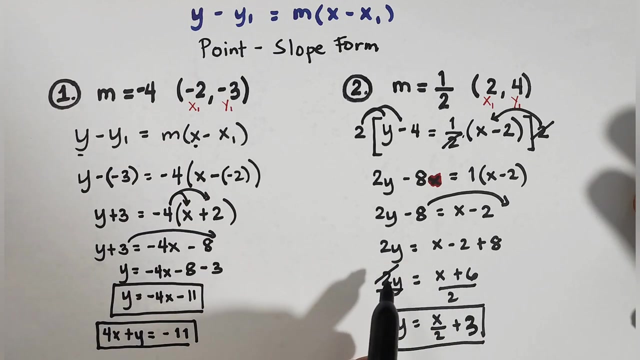 slope intercept form. divided by 2, cancel your y is equal to x over 2 plus 6. divided by 2, which is equal to 3.. This is now the slope intercept form and for the standard form, this is what I will use: The standard form. 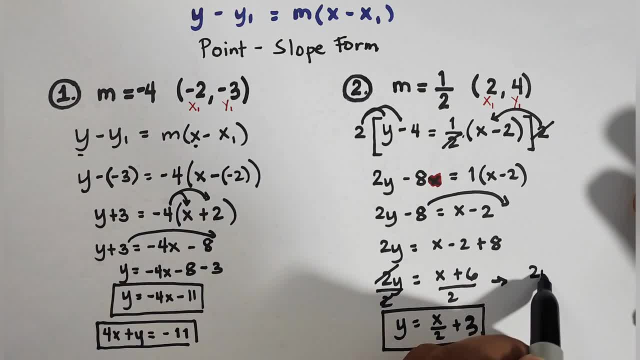 originally we have: 2y is equal to x plus 6.. I will transpose this here. it will become negative: x plus 2y is equal to 6 and then since, as you can see, this is negative, to make it positive kailangan si positive. 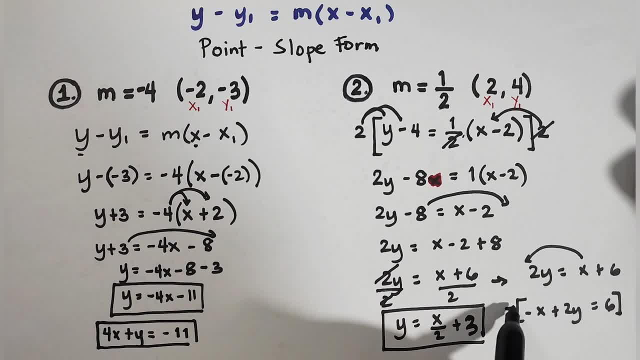 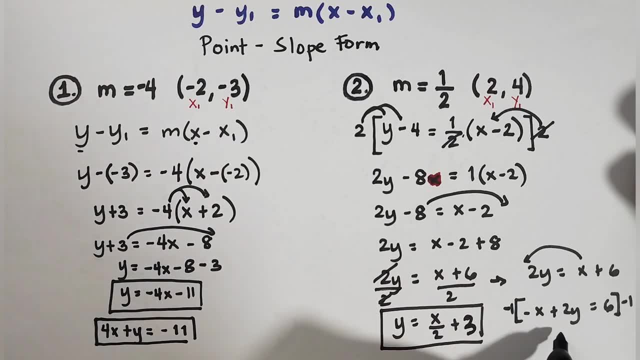 the first term. multiply the location equation by negative 1. so what will happen here? it will change all the sign of the terms. so we have: x minus 2y is equal to negative 6 and this is now the standard form. So I hope, guys, you learned something from this video on how to use the.